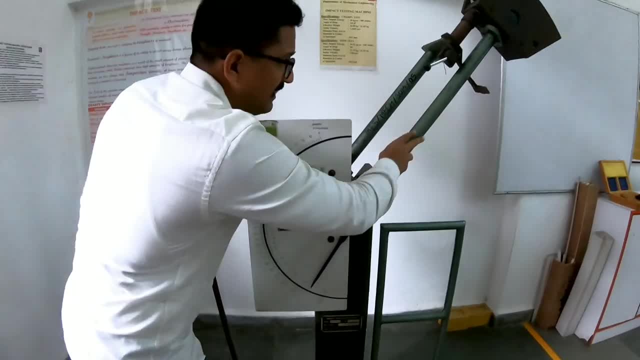 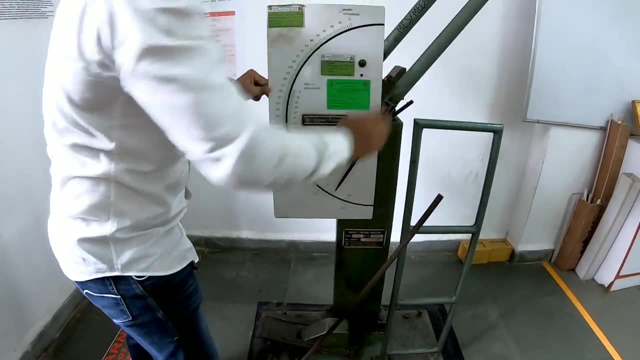 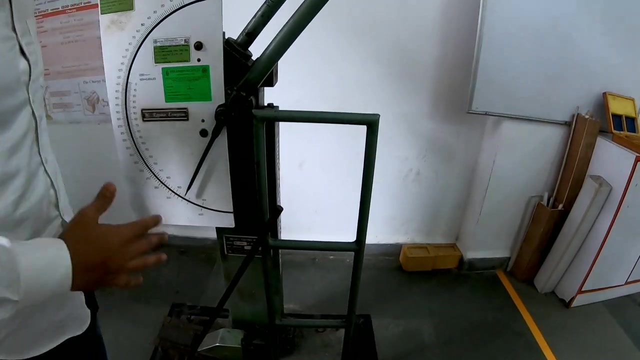 is used to stop the motion or oscillation of the hammer or pendulum. So this stops the swing That we will see in the later part of the video. Then this thing is the safety guard or safety rail. This thing is there to protect the observer or the instructor. 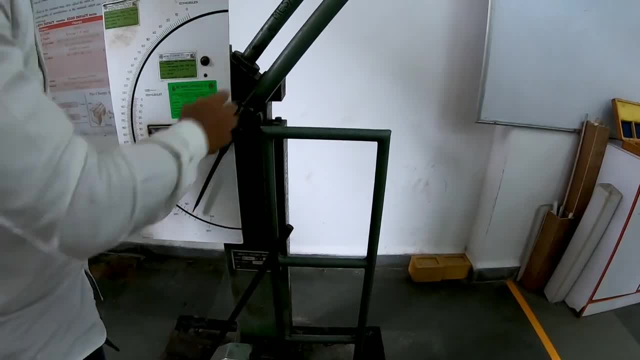 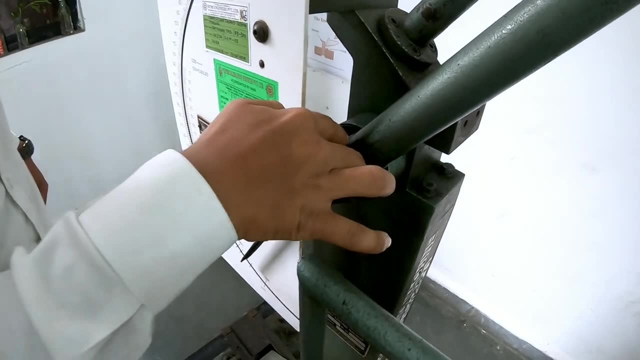 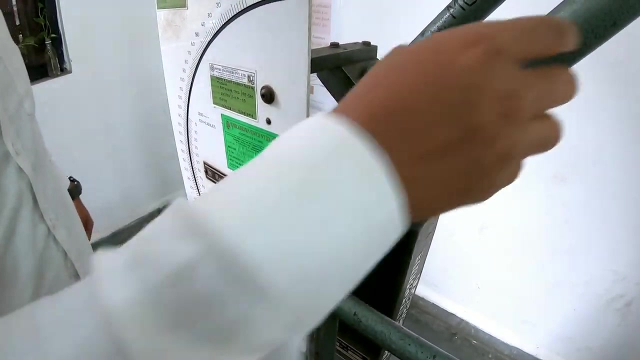 from any damage or to lies, Lost, life and property. This hammer, this hammer, is connected by means of this frame, by means of an anti friction bearing. So this anti friction bearing gives a very smooth flow to the device without any friction or wear. So it is a specialized type of anti. 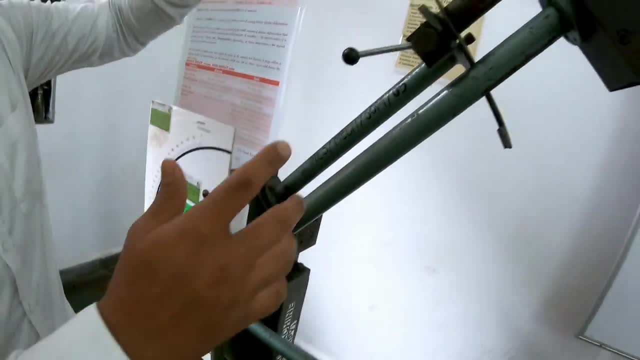 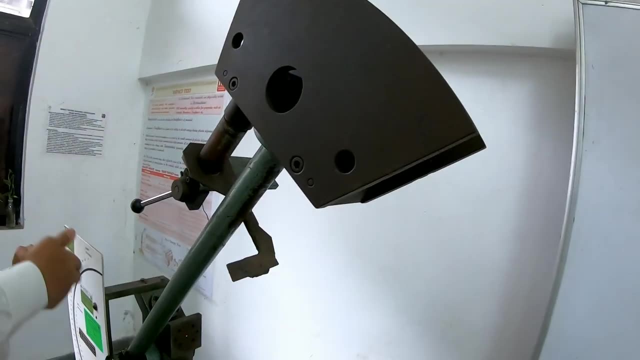 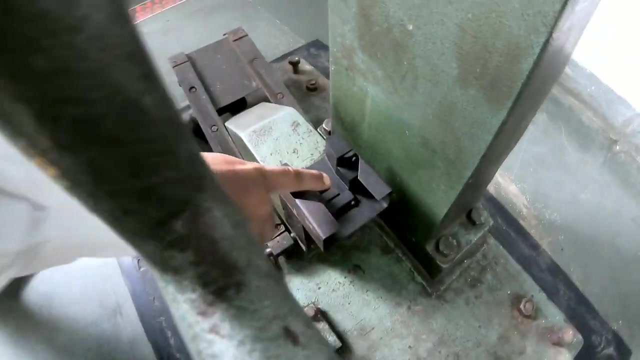 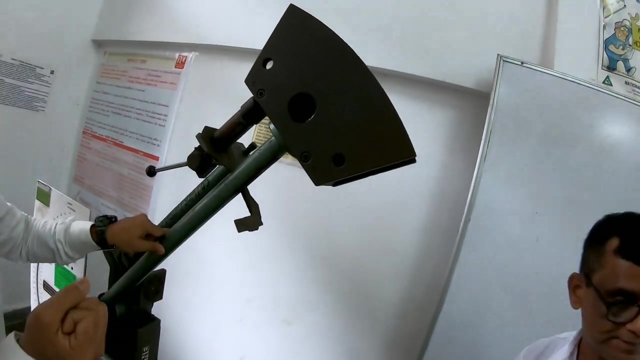 friction bearing which is being used here. Then, coming to the major, important, heavy part of this system, it is the hammer. This hammer basically slides down and hits the workpiece down there, So the workpiece is stationed here, and when the hammer falls from this height to the workpice, it gets absorbed, the energy. 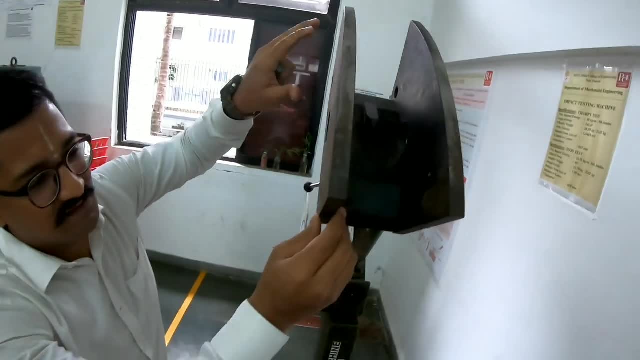 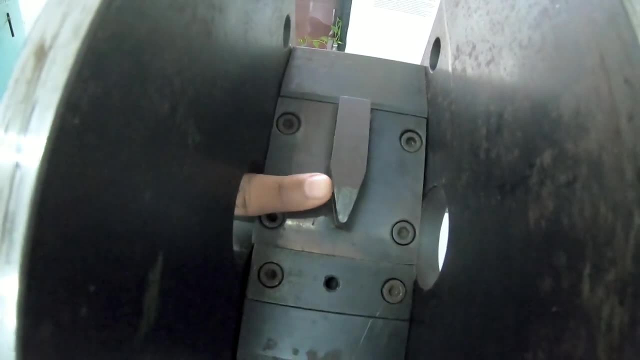 which is our final aim. So this hammer consists of a- you can see striker. there on the center There is a striker. This striker is basically a nose head type striker. This striker is a type of striker, actually a light striker. It is kind of big. They arebeing designed to make it look like 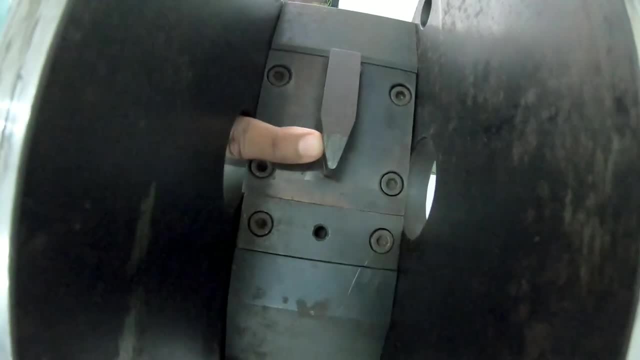 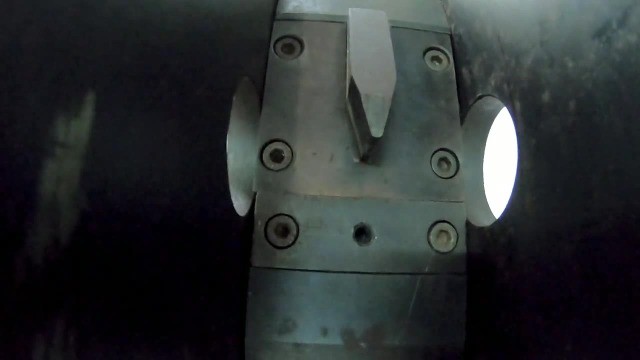 a striker. It is in that, you know, in this camera, a striker. they are getting hit as striker. the shape of the striker is nose, head, and there is a angle to it, given to it angle. this angle is the angle of the striker. all these are standard equipments which are used. 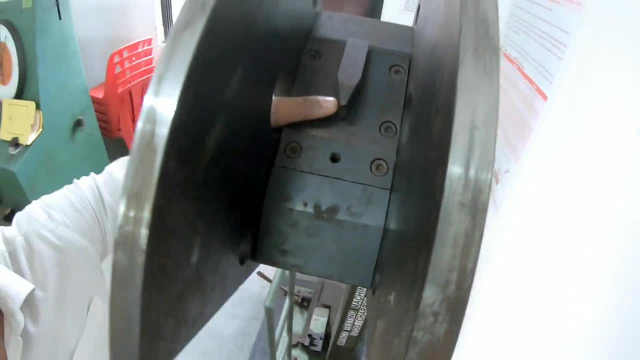 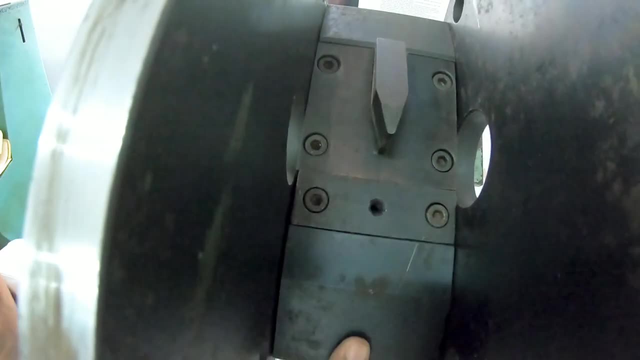 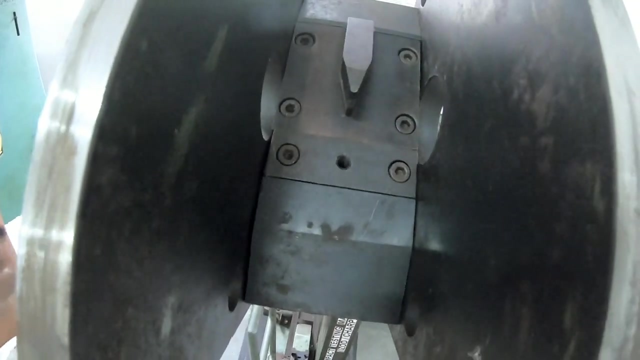 for charpy test. another example which i will show you about the striker is and the. the material for this striker is high carbon steel. as we know, high carbon steel is a very tough material and the material which we are using at the work place is mild steel, so this material- 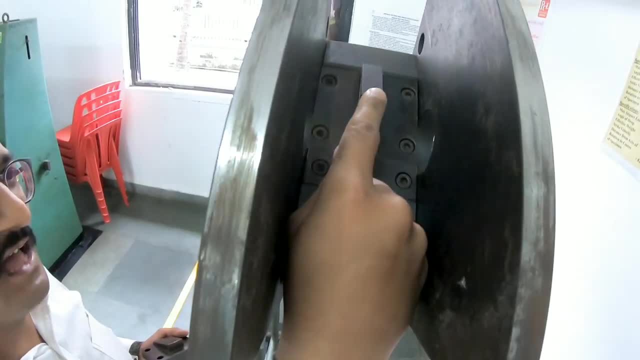 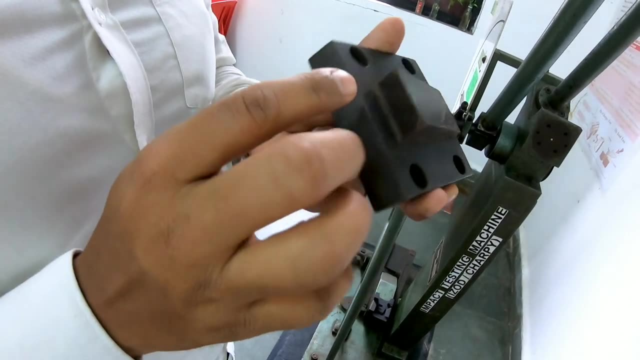 should be tougher than the specimen which we are using. so this is a high carbon steel. you can see here that this is a another striker which i am showing you. this striker is used for izod testing, which will show, which will see in the later part of the video. today we 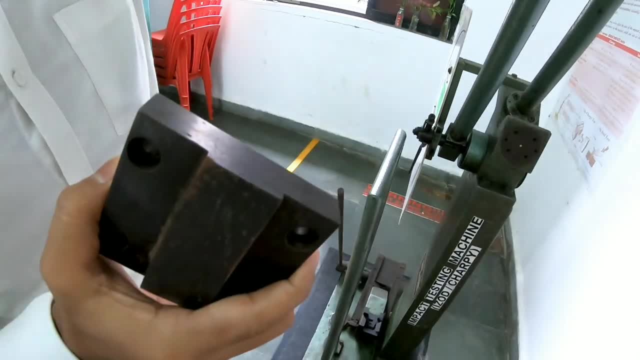 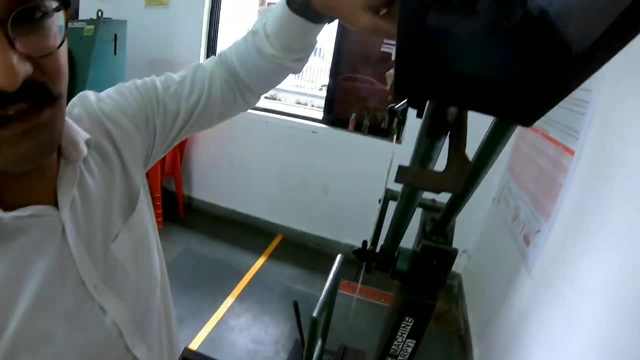 are performing charpy test. so it is a nose head type striker. this is a flat, flat head type striker. you can see the shape of the striker is flat head and in here it is a nose head type striker. so this is all about the hammer and its striker. 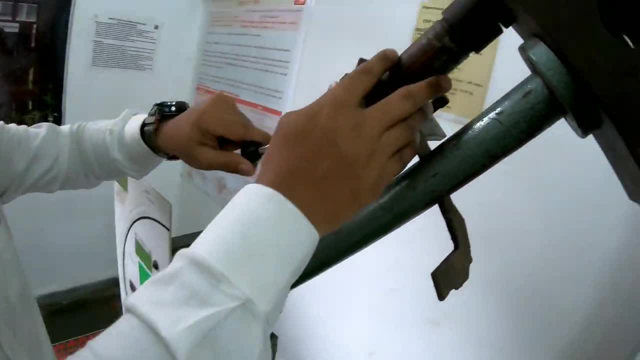 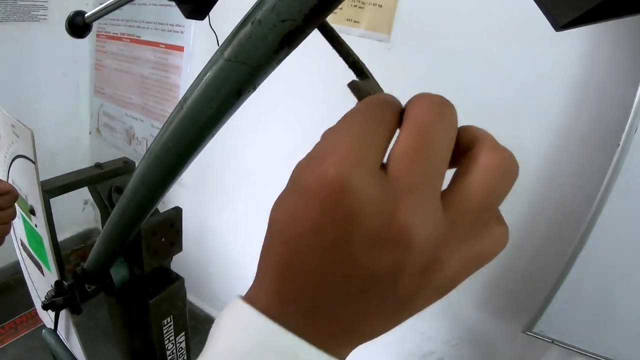 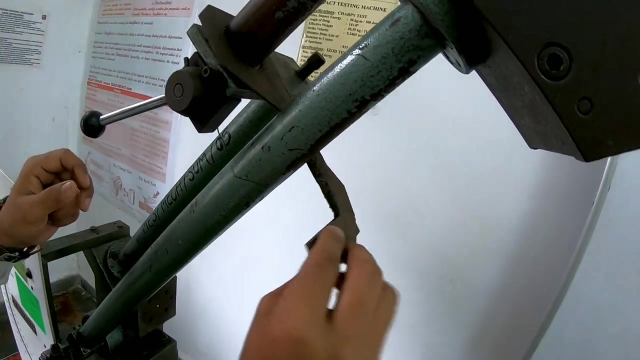 part. this is the latch, this is the latch part and this is the release valve. when i release this valve, this hammer will go down and this is a safety latch we can say for extra precaution if, by mistake, if i release this valve, so it will help this hammer to lock it down. so this: 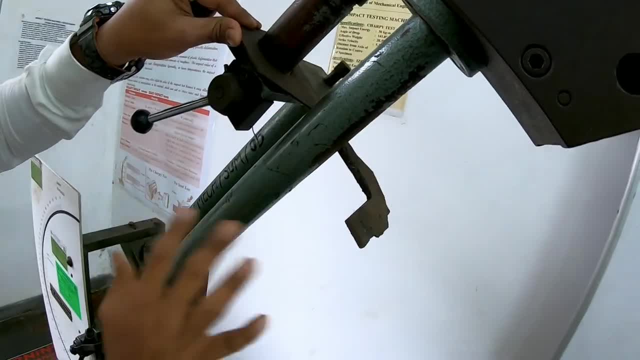 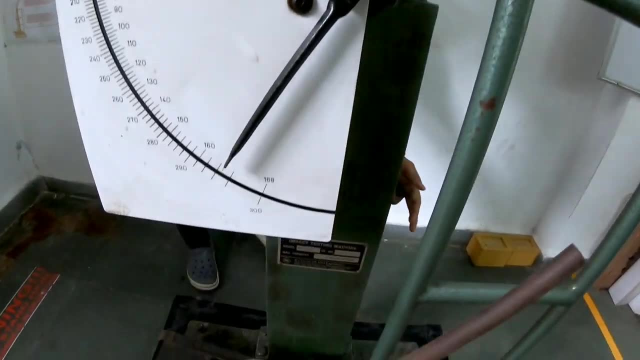 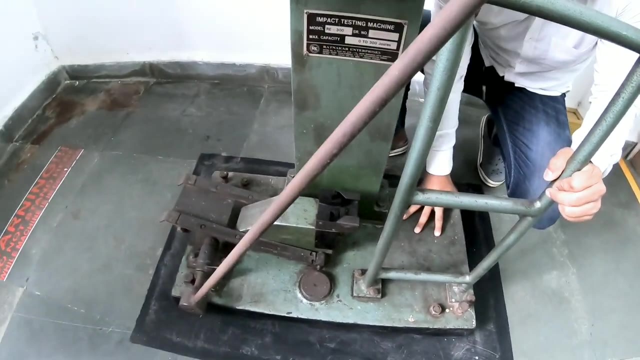 is a specialized extra protection which is given to this equipment. now, this is the frame here. this is the frame. you can see. this is the frame and very rigid foundation is given to the setup. why this rigid foundation is needed? because no vibration should be there in the system. that's why this rigid foundation is. 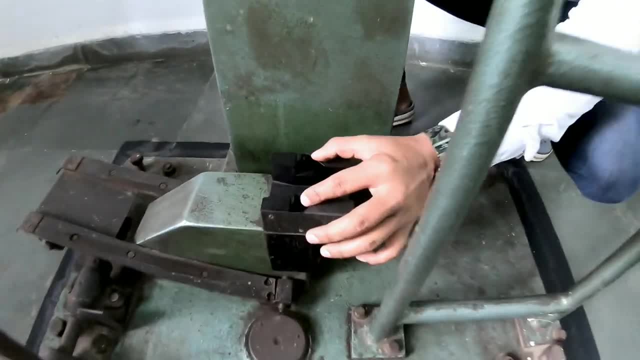 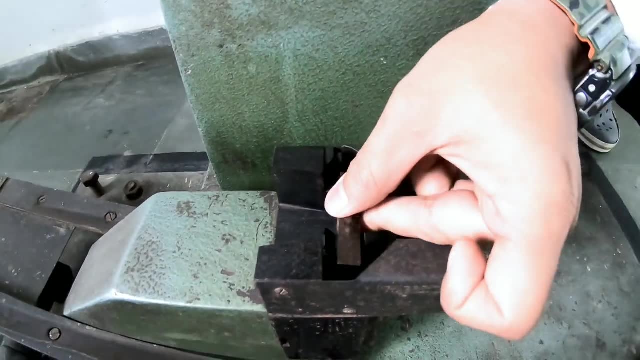 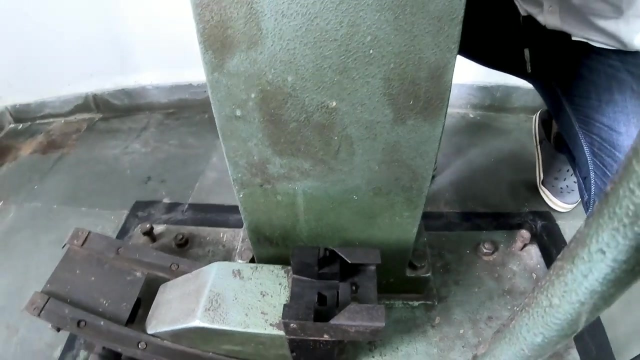 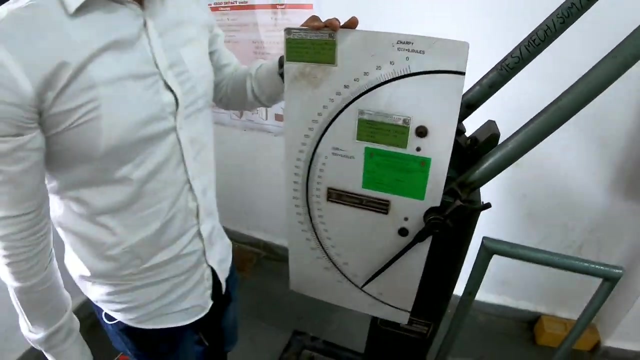 being given. this is the part where the work piece is held for this experiment. it is called as anvil. so here the work piece will be placed, something like this, and when the striker hits it it will get break, or the total energy absorbed by the material we get in the dial. so this is how. this is how the setup of the charpy test is done, and 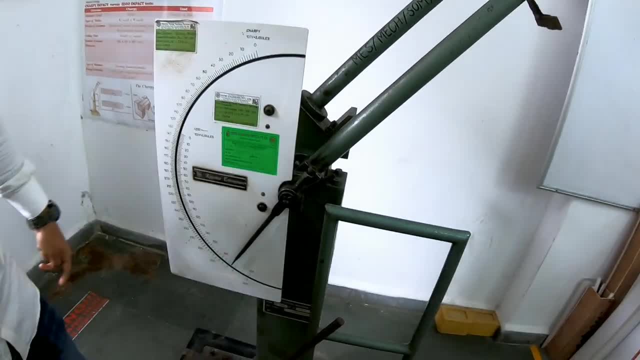 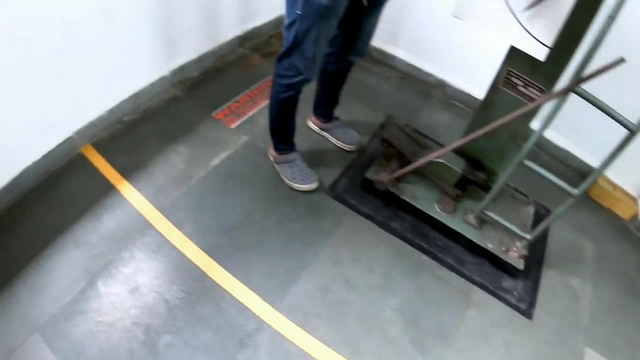 before going into the test. and this is this part, this yellow part. you can see this yellow part. this yellow part is the region in which no student or no instructor should come or cross this boundary. so this is the yellow part. this yellow part is the region in which 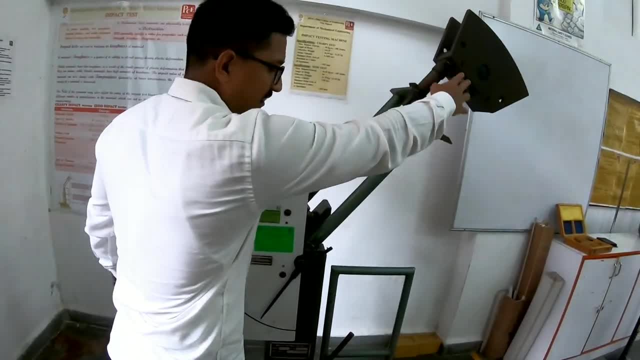 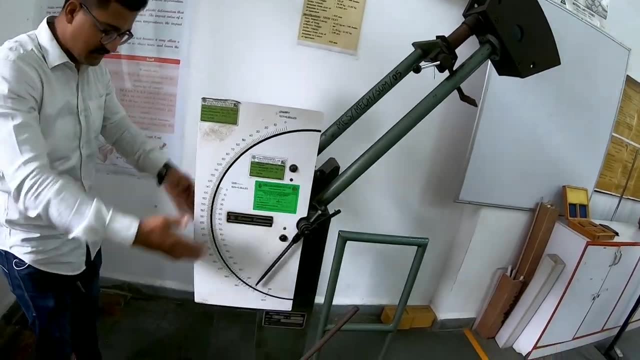 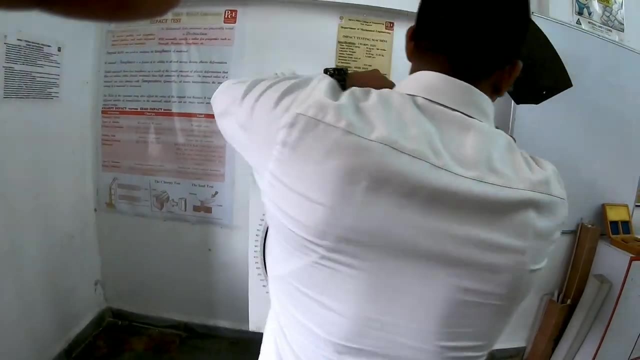 no student or no instructor should come or cross this boundary, because this hammer is having a lot of weight and it will be very dangerous if this somehow, if this will be released and someone is standing here, so it will be directly hitting the person and it will be very bad face for the instructor. i will show you that why it is important? because 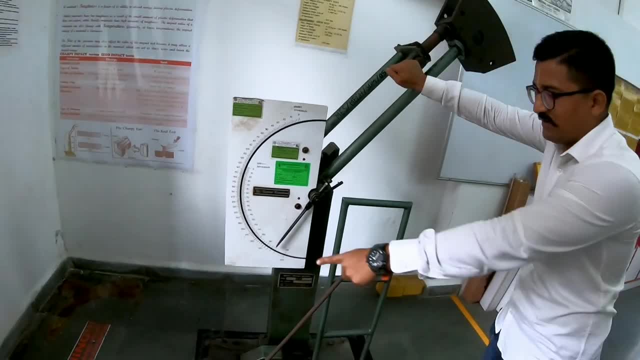 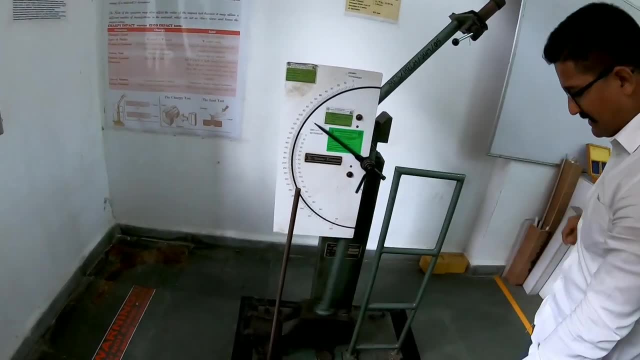 if you release this, you can see, if i release this wall and someone is standing there, you see it will hit that person. so that's why it is very dangerous to come inside the wall, because this wall is very dangerous. so this wall is very dangerous. so if you release this, 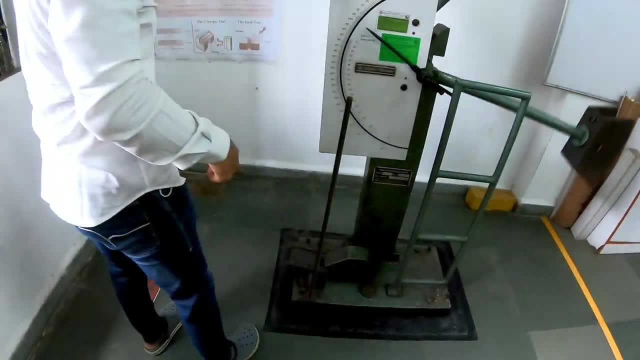 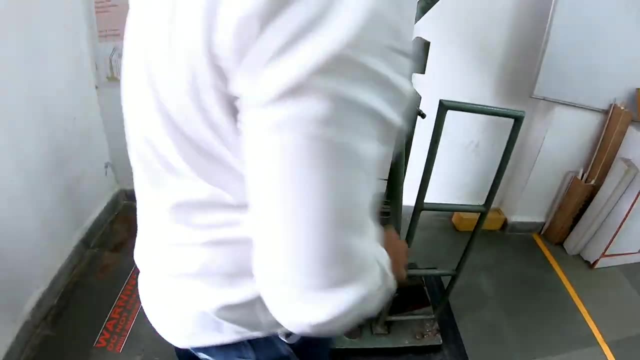 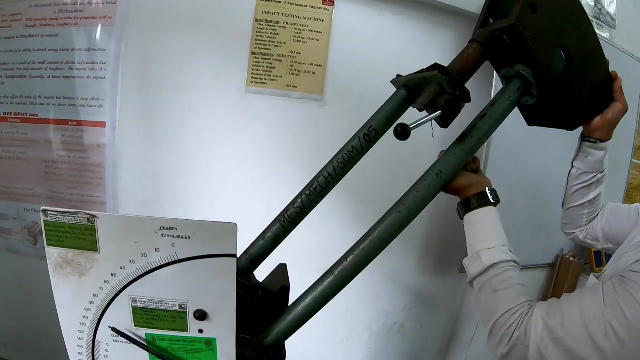 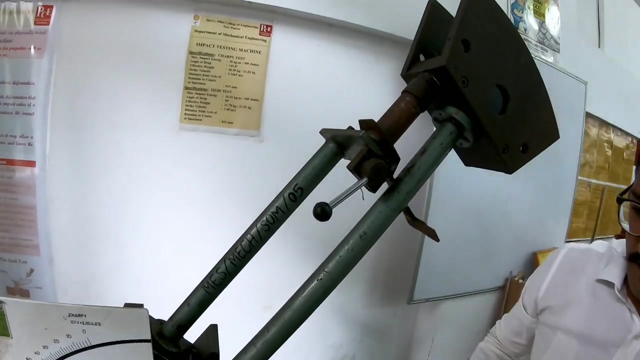 inside this yellow zone and we can stop this device by means of this mechanical brake. so that's why the mechanical braking is provided here. you can see, now I will perform this test for you. so now this again will perform the test. so now, before going into the test, I just 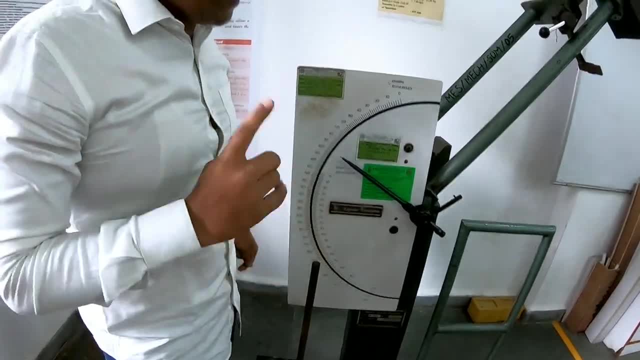 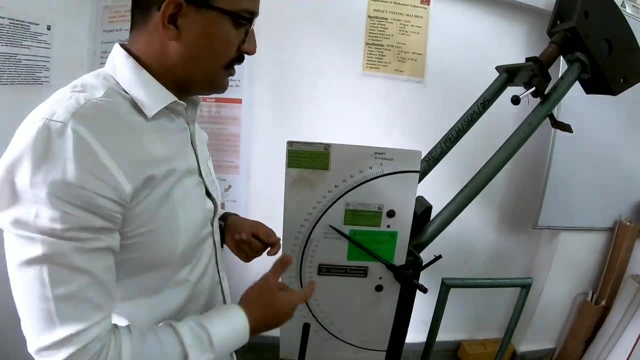 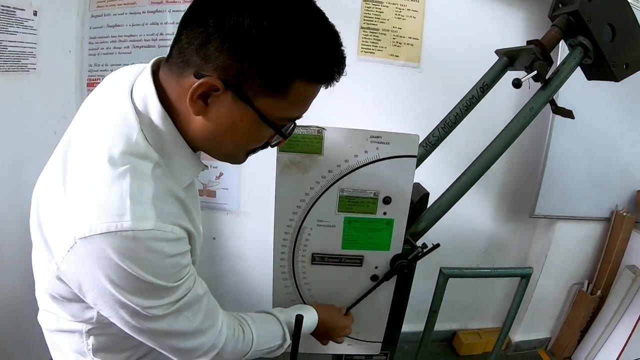 want to show you that we will perform this test, this sharpie test, first without the specimen and then we will perform the test with specimen. why without specimen? to check the calibration of the instrument. we are performing it first without the specimen, so without the specimen first. I will keep the pointer at the maximum, since this is a sharpie scale which we have. 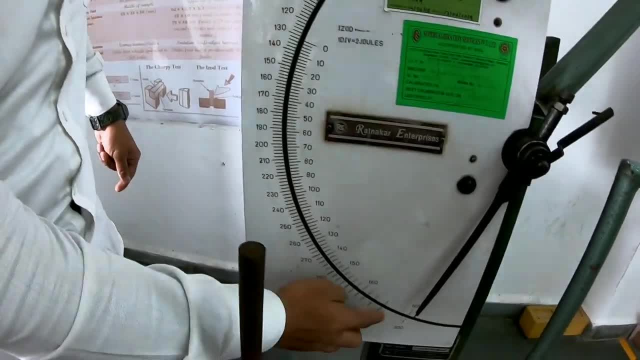 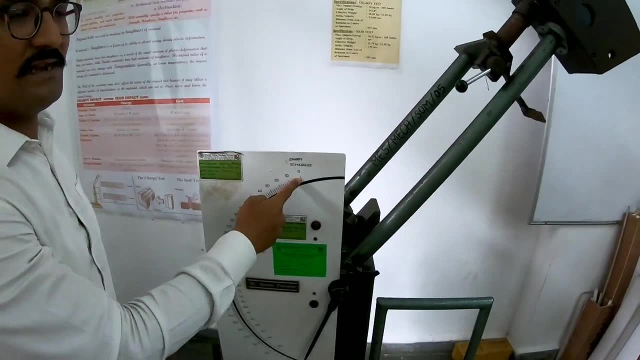 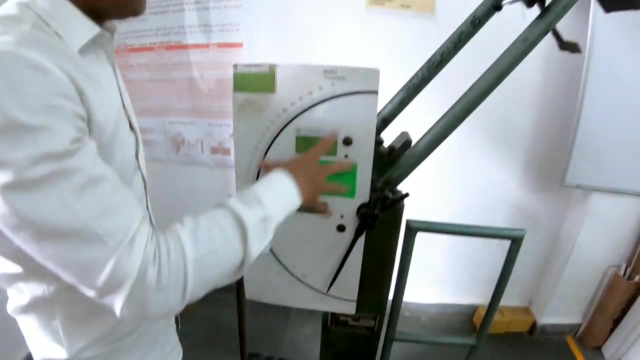 to consider the outside one, as I have already told you in the video. so I will keep it at the maximum. so I will keep it at the maximum and then I will perform the test with the specimen. And when I release this valve, the reading should be zero. Correct. Why the reading should be zero? Because there is no specimen there, So no energy is absorbed by the system. So that's why it should get a zero reading, Correct. 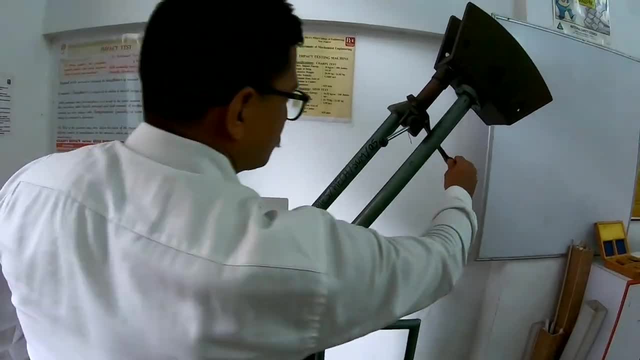 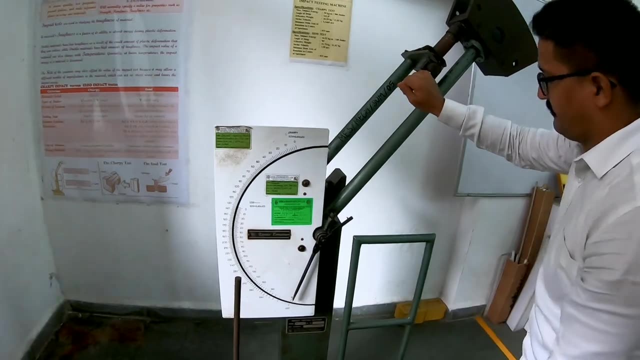 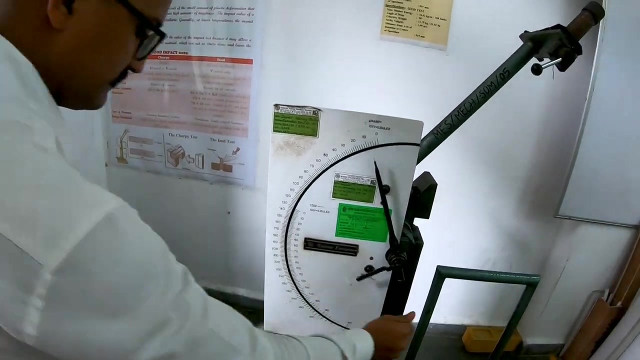 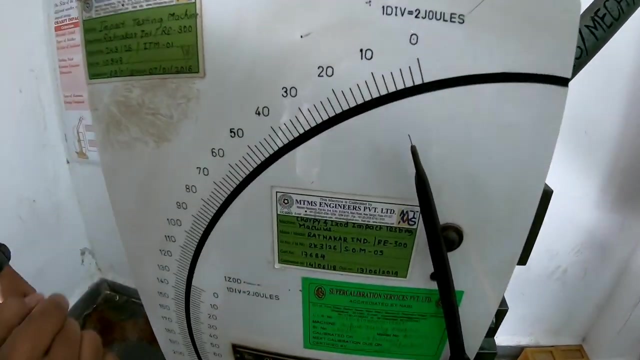 So let us see whether we get the zero or not. We have to take all safety measures. Now I will release and see the reading. So now I will apply the mechanical braking So you can see here now on the reading that it has not come zero. It has been around 8 joules. So why this error is there? 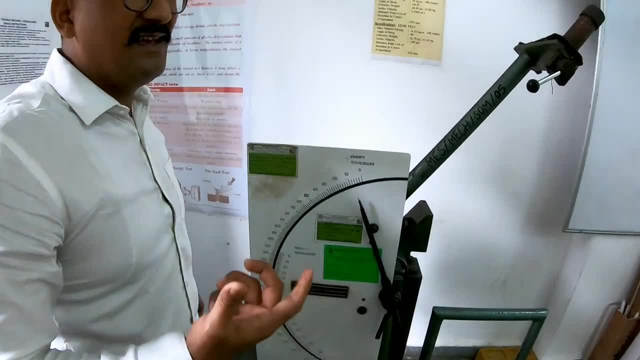 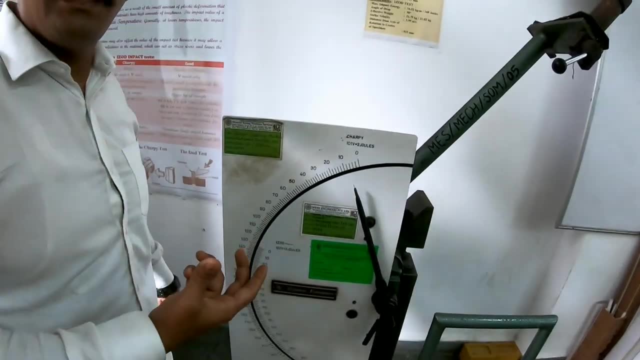 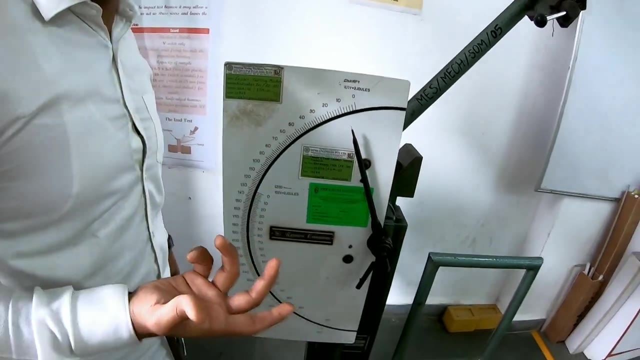 So this error is there. there may be, for due to some. you can say you can see that the friction is there in the instrument and then some human errors are there and some technical errors are there. so this 8 joules, you can account for some errors in the system, which is quite obvious. 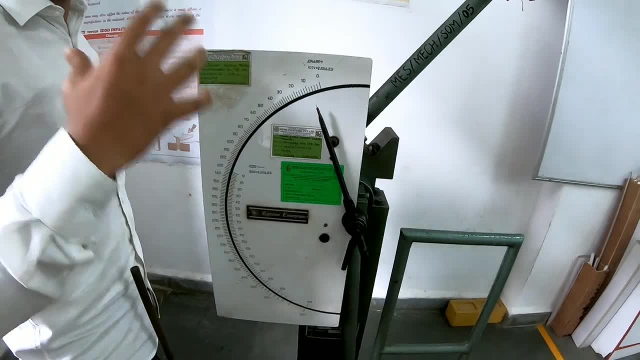 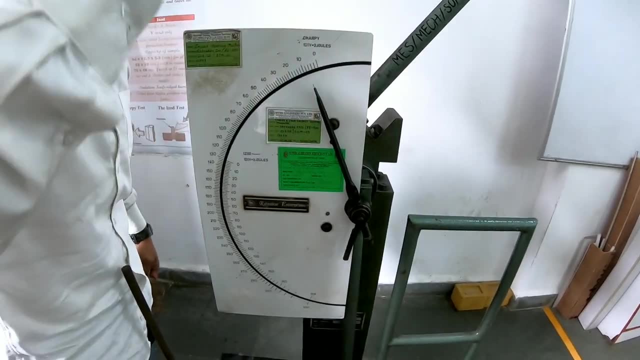 which will be there, but for the real time conditions, or for actual condition, it should be around 0. so what we will do? this 8 joules we will minus from the actual reading during the final reading this 8 joules. why we are reducing this 8 joules? because it is a error. 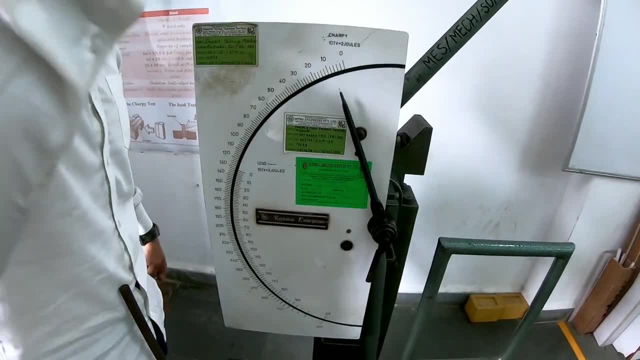 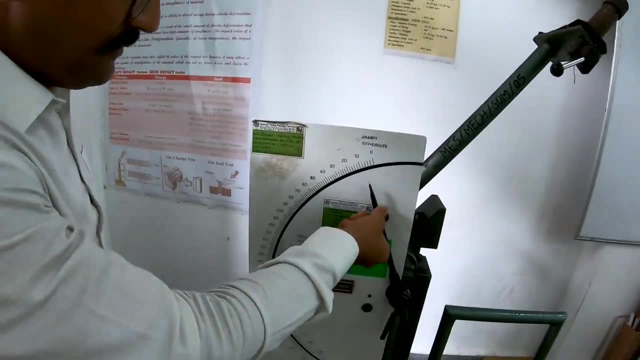 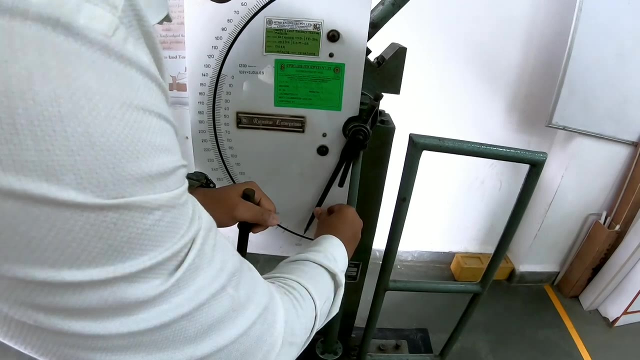 so we will reduce that error by taking into account this error during the final reading. so final reading minus initial reading will give you the exact reading, correct? so now we will perform this test by help of a specimen, correct? so this is again the 0th maximum value. 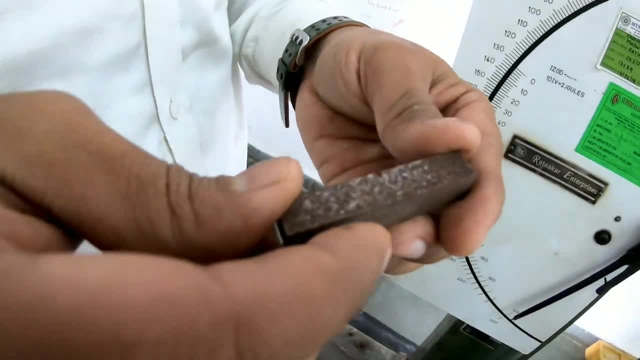 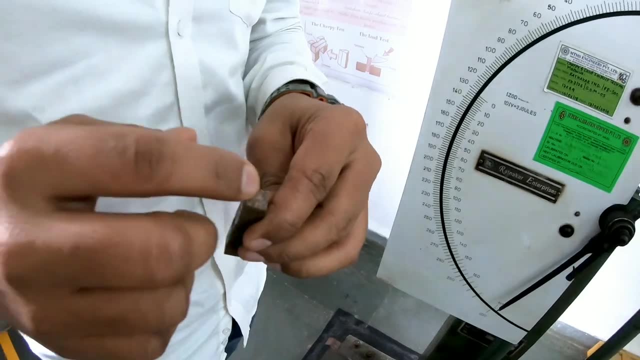 and this will be for iso test. Now, this specimen we are going to use today for doing the charpy test, the length is 55 mm and the cross section is 10 by 10, 10 by 10 and we will place it. patinser will place it here. 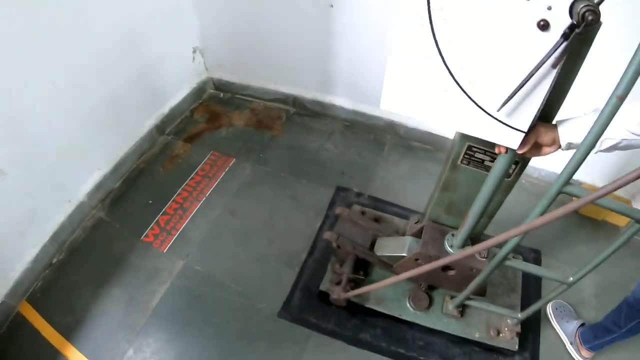 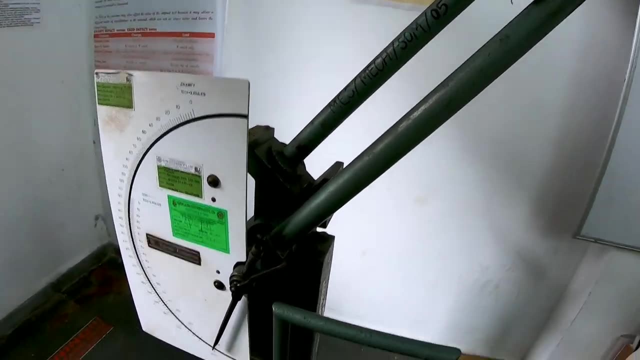 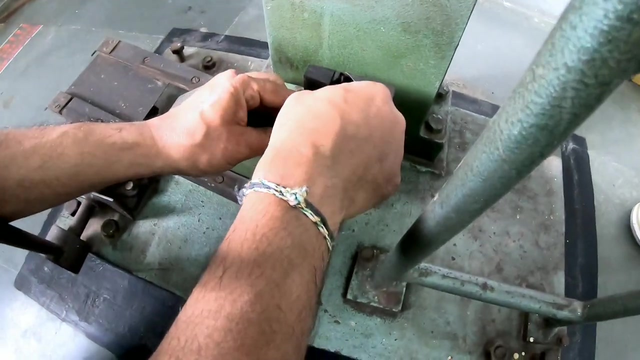 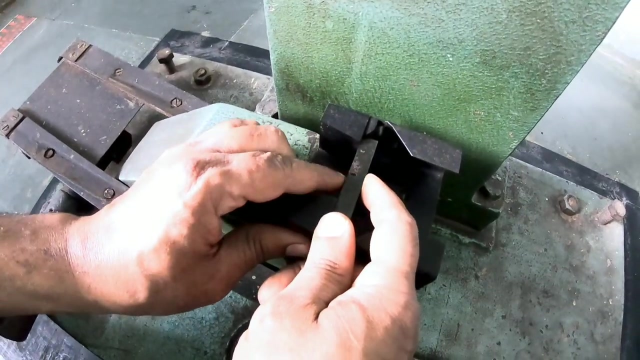 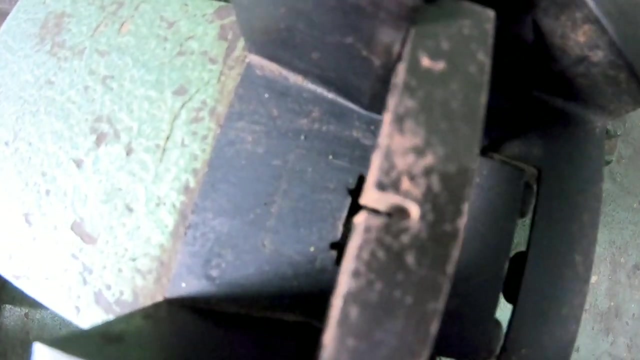 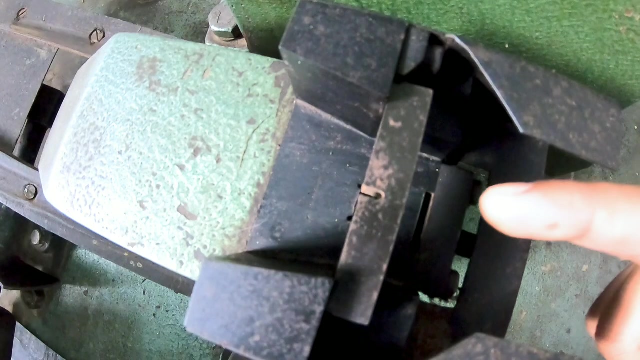 so you can place that we will again. so patinser is now going to place the specimen there on the anvil. This is how the material is placed on the anvil for the charpy test. the main important thing is the notch should be opposite to that of the striker. the striker will hit somewhere. 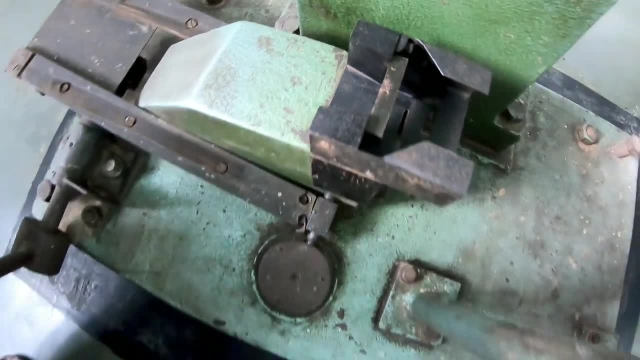 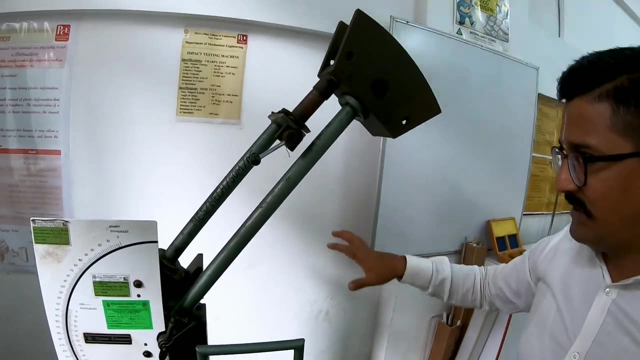 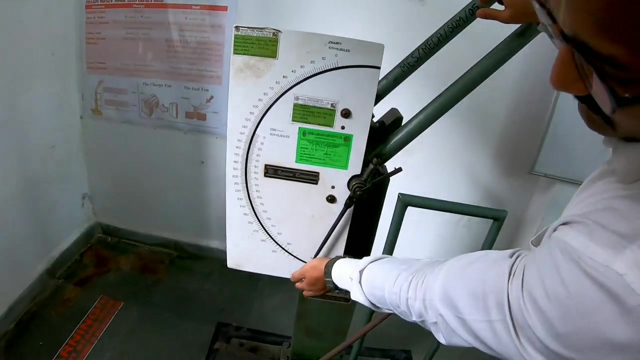 here and the notch is opposite to that. so this we have to take care of. Now we will perform this test. we have to be extra cautious about this test because the warning is already been placed there, so now i will. i have kept the pointer at the maximum and 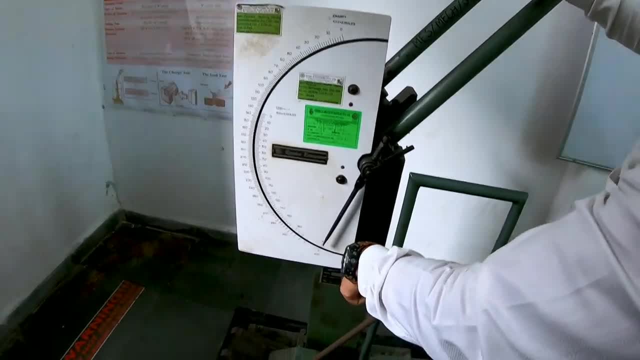 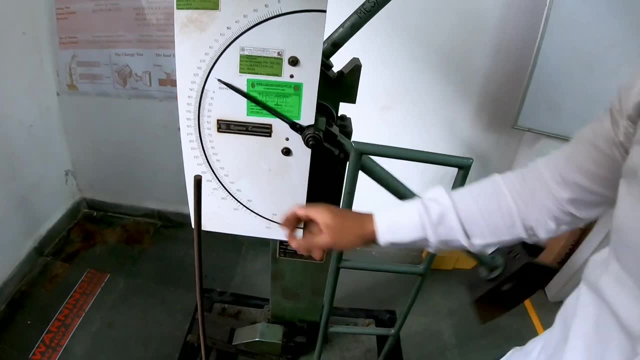 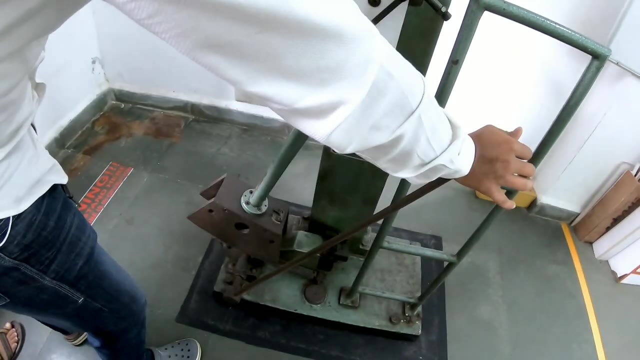 we will see how much energy is absorbed by the material, by that mild steel material. in terms of the reading, now i will release it. you can see. so the material has been distorted and now i will stop this by means of mechanical braking. now you can see that the nature of 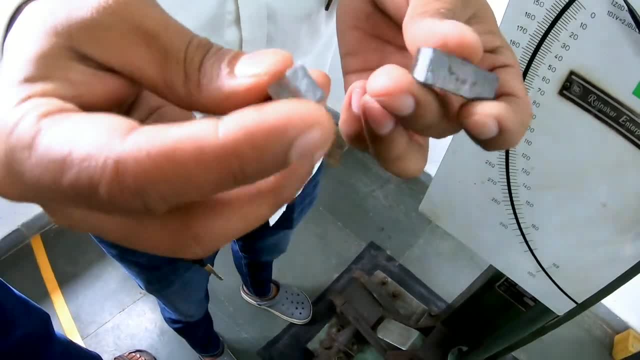 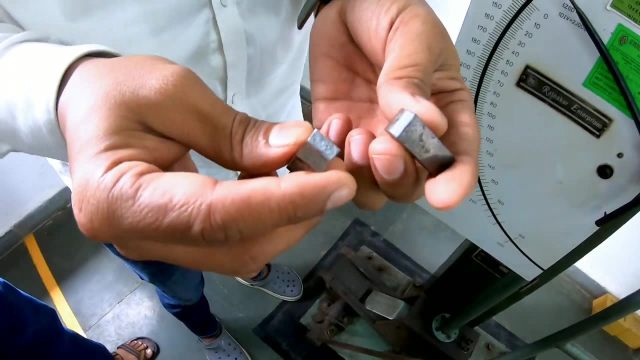 the failure of the material. you can see the total energy absorbed by the material is somewhat like this. you can see the failure pattern. because of the impact energy absorbed by the mild steel model, it got broken down into two pieces, so you can imagine the type of energy.